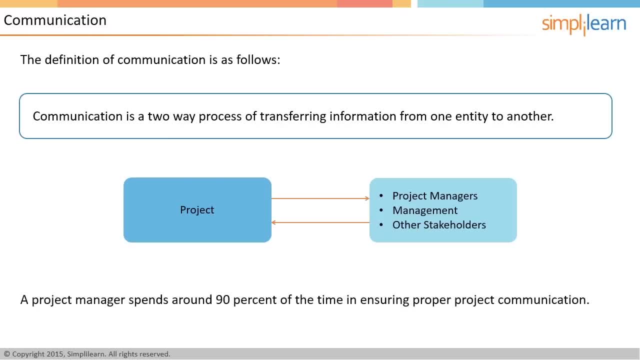 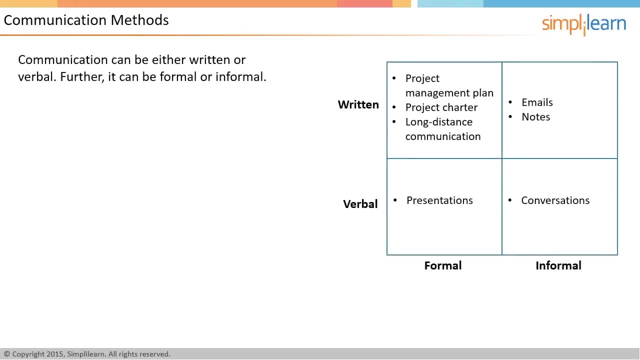 for ensuring proper communication to and from the project. In fact, a project manager spends almost 90% of his or her time on communication. You can now understand how important it is for a project manager to plan this activity well. In the next screen, let us discuss communication methods. Communication can. 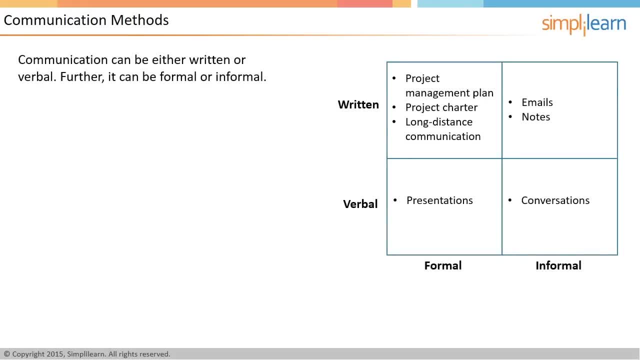 be done in two ways. It can be done written or verbal. Both written as well as verbal communication can either be formal or informal. Formal means communicating by following some basic rules, whereas informal means taking a casual approach. These two combinations result in four different communication. 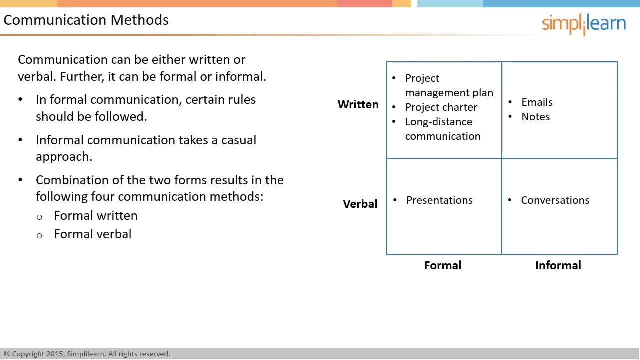 methods. They are the following. The first is a formal communication, where the They are formal, written, formal verbal, informal written and informal verbal. Formal written method is used for project management plans, project charter and over long distance communication. Formal verbal method is used during presentations, whereas informal written method is applicable. 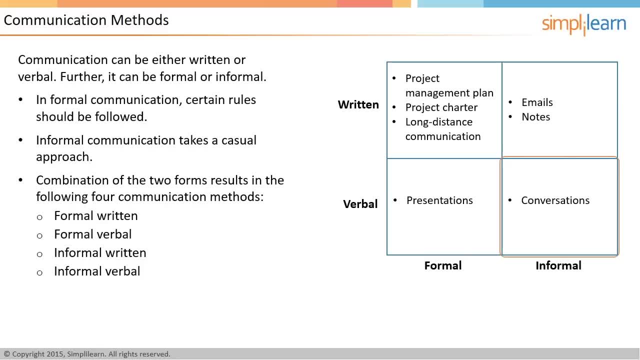 while writing notes or emails. Informal verbal, on the other hand, is applied during conversations. You can expect questions in the PMP exam which require choosing a communication method for a given situation, so a fair understanding of the communication methods can help you. 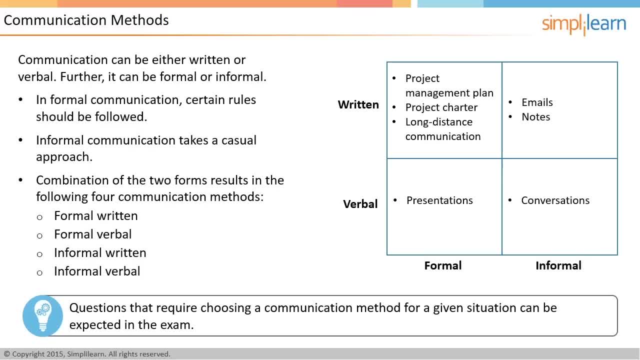 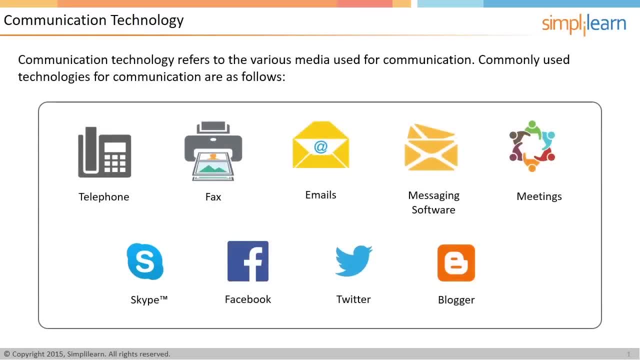 score higher. In the next screen, let us look at the various communication technologies. Communication technology refers to the different media used for communicating. A few such technologies are listed on screen, among which email, fax and telephone are available. A few popular communication technologies. 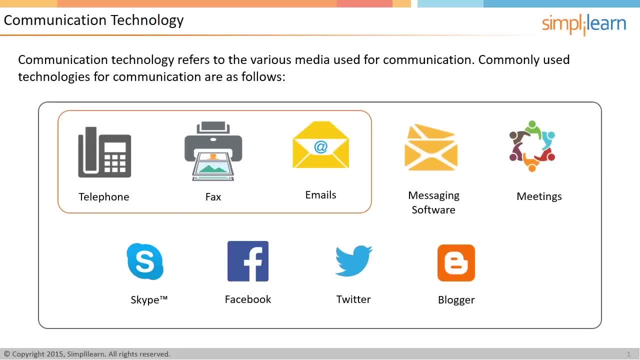 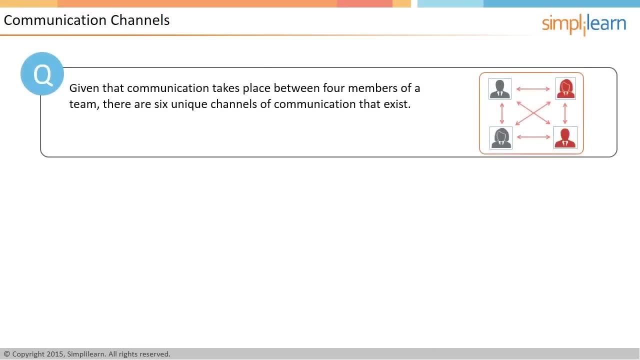 In the next screen. let us understand the communication channel with the help of an example. Communication takes place between four people in a team. The lines across the members represent there can be six unique channels of communication existing within the team. Now, if the team comprises ten members, how many unique channels of communication will? 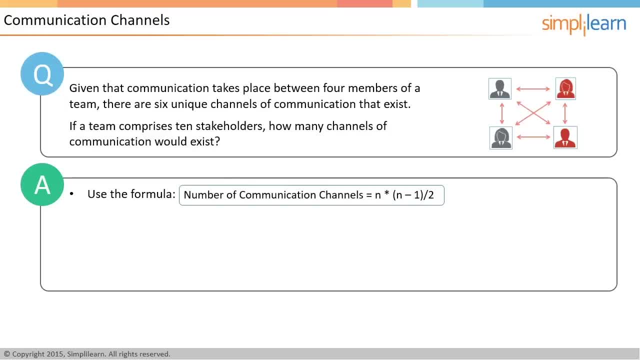 be calculated. You can use the formula. N is the total number of people involved in communication. in this case, N equals 10.. If this is put into the formula, you will get 45 as the result. Therefore, 45 unique communication channels exist in a team of ten people. 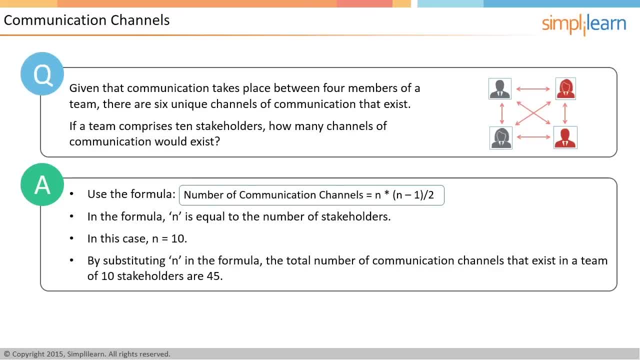 It is difficult to manage such a large number of communication channels. Therefore, it is important to know how many unique channels exist in a team of ten people. You can use the formula to calculate the total number of people involved in communication. It is important to structure communication. 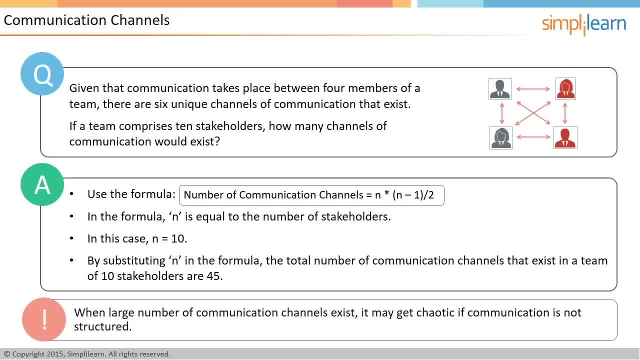 Otherwise everyone starts communicating everything to everyone and it can become a real chaos in the project. In the PMP exam you may be asked to calculate the number of communication channels in a scenario-based question, so please make a note of the formula to answer the question. 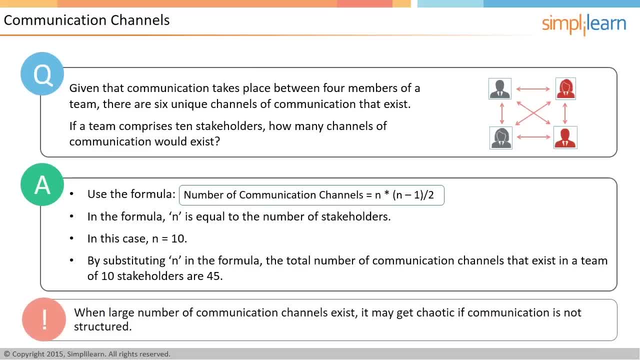 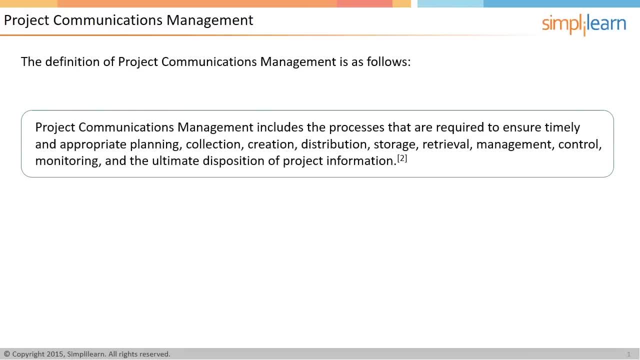 correctly. In the next screen let us discuss the basic communication model. Project communications management includes the processes required. It is required to ensure that information about timely and appropriate generation, collection, distribution, storage and ultimate disposition of project is prepared and circulated. 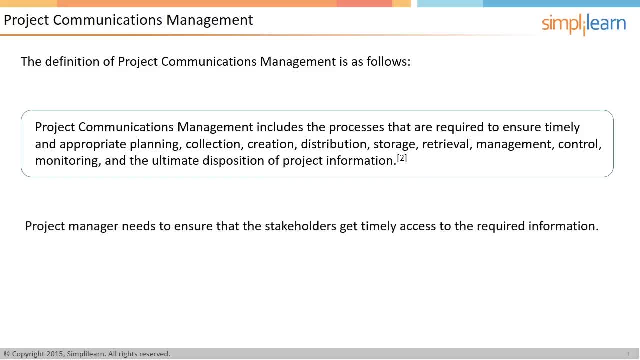 to all project stakeholders. It is the responsibility of a project manager to ensure that the information requested by the stakeholder is communicated to them. The frequency at which the information needs to be shared may also vary from stakeholder to stakeholder. For example, think about a simple process of sharing a project status report with the. 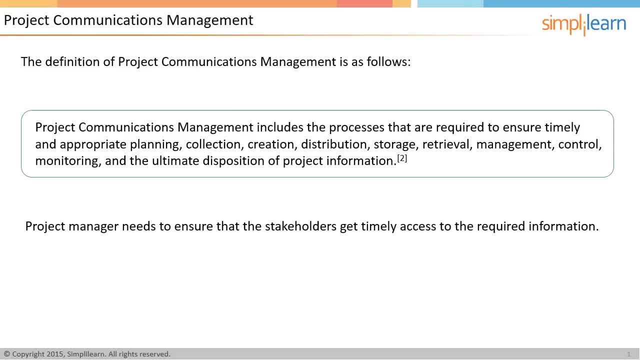 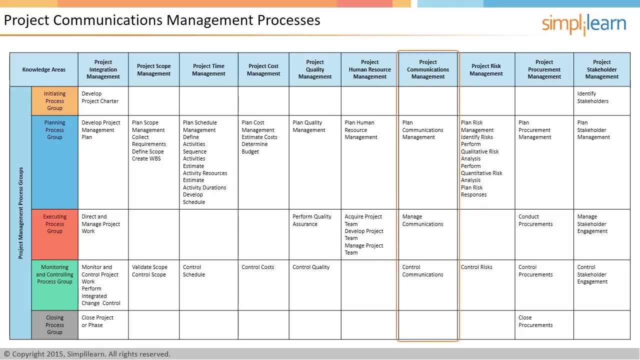 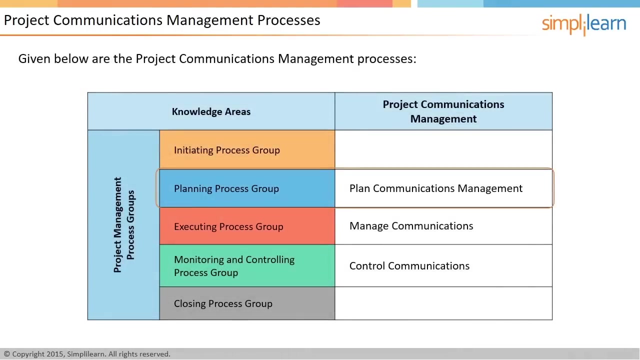 customer and senior management. This knowledge area explains how it should be done as per PMI. In the next screen let us discuss the project communications management processes. There are three project communications management processes. Process is carried during different process groups. Project communications management is done during planning process. group manage communications. 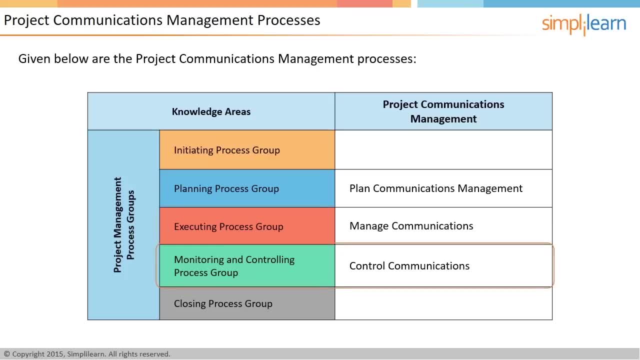 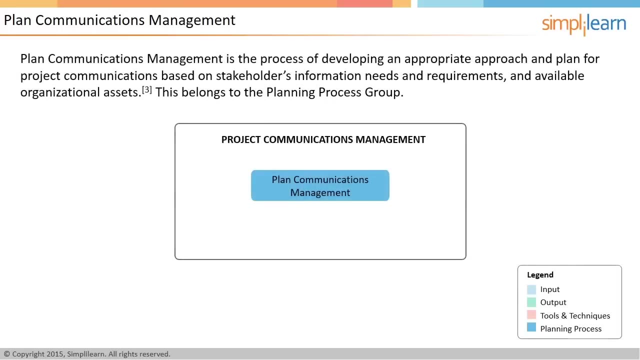 is done during executing process group and control communications is done during monitoring and controlling process group. In the next few screens we will cover each of these processes in detail. Plan communications management is the process of developing an appropriate approach and plan for project communications based on stakeholders' information and the project's. 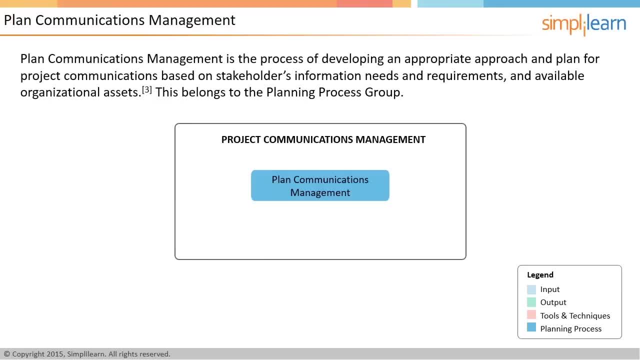 information, needs and requirements and available organizational assets. This belongs to the planning process. group Stakeholder register is an important input to this process. It is a list of all the stakeholders. The project management plan has information about a large number of the project's requirements. 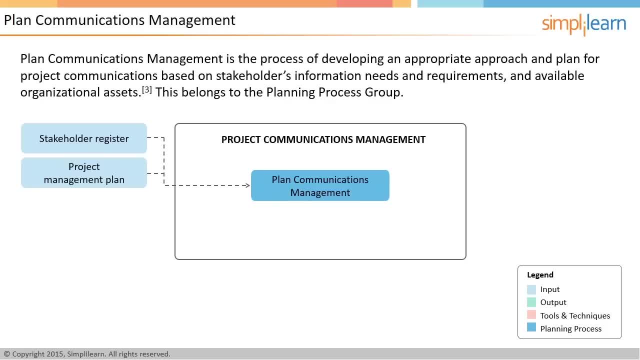 and the stakeholders who need to receive communication of various kinds are therefore a critical input to this process. In addition to these two, organization process assets and enterprise environmental factors are also inputs to this process. Many organizations have standard templates to prepare communication management plan. 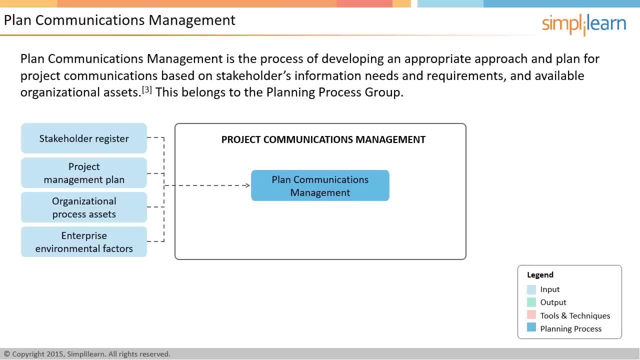 which are part of the organizational process: assets and enterprise environmental factors. The first technique used in this process is the communication requirements analysis. The first technique used in this process is the communication requirements analysis, Where the communication requirements of each of the stakeholders are analyzed and categorized. 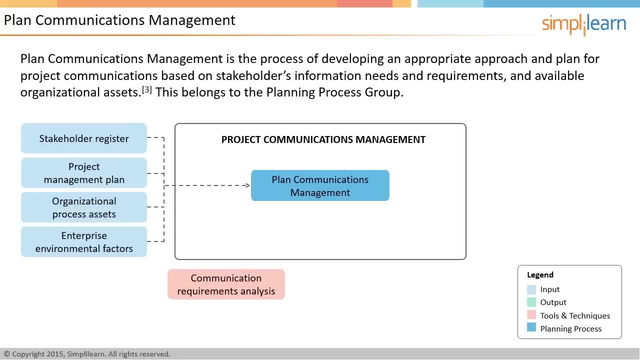 In this you try to find how many of the stakeholders need similar kind of information which can be grouped together. If you send information through an email system, all those stakeholders who need similar information can be marked in CC in the email. Next you can decide on the communication technology. 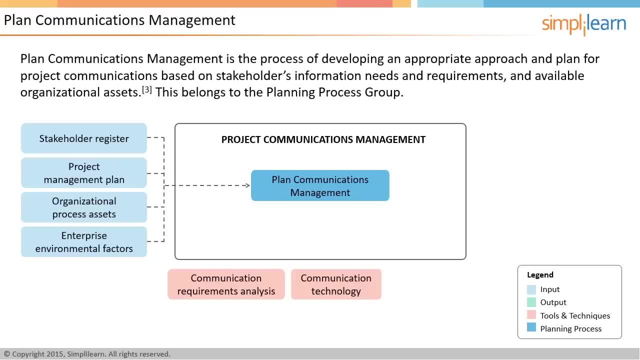 These days, email is the most widely used technology. It is the most widely used technology in the world, But in few cases you might have to send information using some other technology, like fax or registered post. For example, all government communications are done using registered post to keep a written. 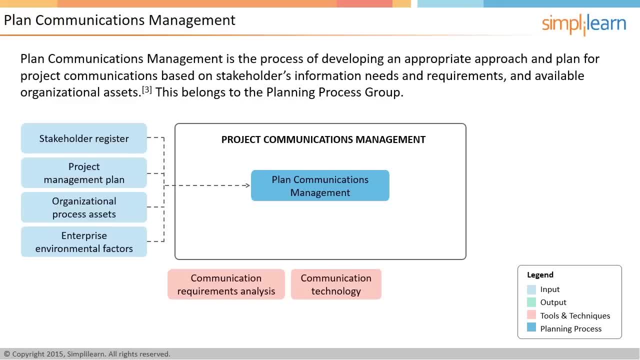 record. Finally, you need to understand how communication really happens, That is, the communication models and the various communication methods used. You may need to conduct meetings before agreeing to continue the communication process. If you need to know about the communication plan and how it works, you need to know the 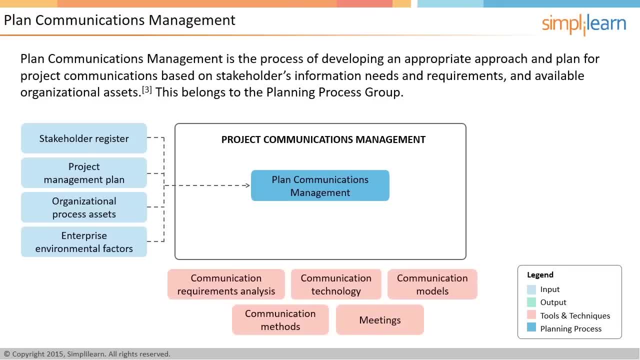 before agreeing on and finalizing the communications management plan. The communications management plan is the primary output of this process, which lays down the procedures around communications in the organization. Communication management plan has information like which stakeholder needs what kind of information, at what frequency and how. 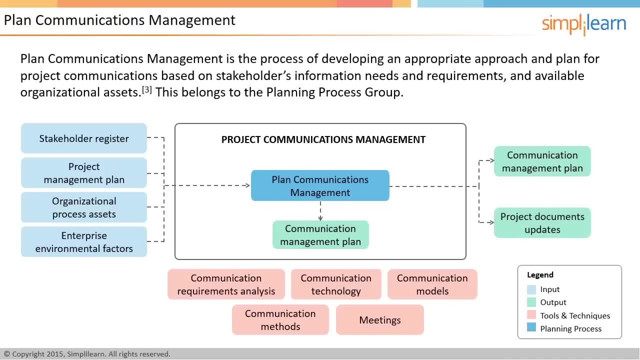 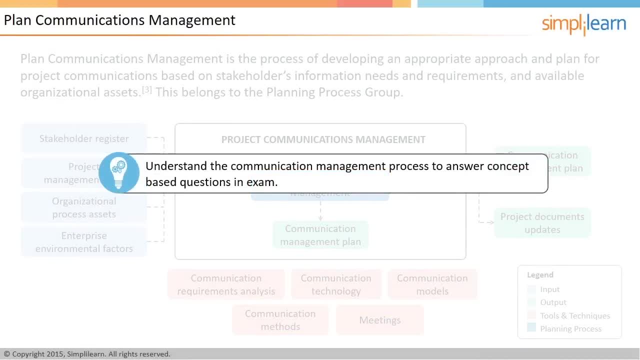 As a result of this process, some other project documents may also get updated. There may be questions in the PMP exam based on the plan communications management process, so a fair understanding of the process will help you answer such questions correctly. In the next screen, let us look into a business scenario to understand this concept better. 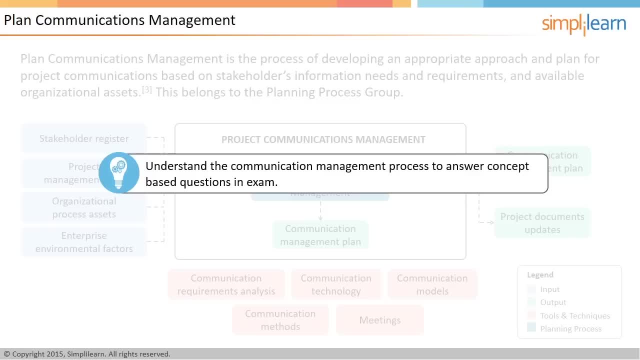 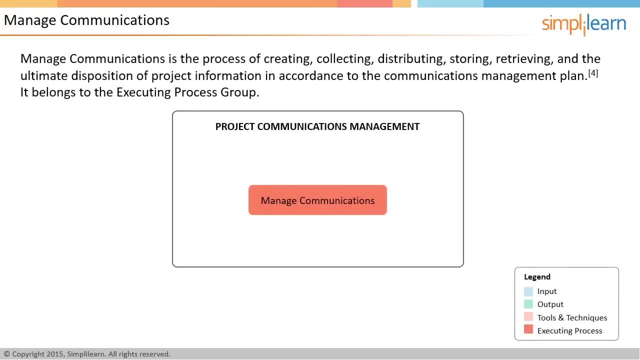 After reading the problem statement, click the solution button to look at a possible answer. Manage communications is the process of creating, collecting, distributing, storing, retrieving and the ultimate display. Manage communications is the process of creating, collecting, distributing, storing, retrieving and the ultimate display. 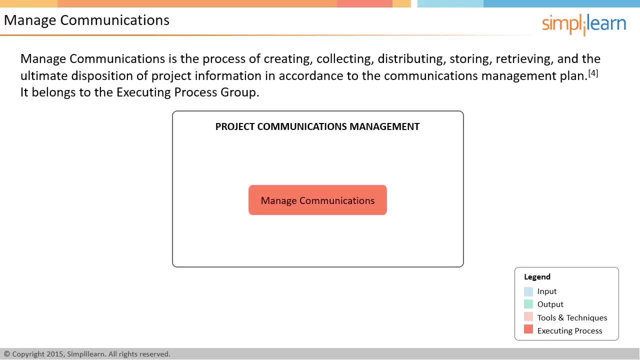 Manage communications takes care of the composition of project information. in accordance to the communications management plan, It belongs to the executing process group. Manage communications is done throughout the project lifecycle. Everything cannot be planned during communication planning, so manage communications takes care of responding to unexpected requests for information as well. 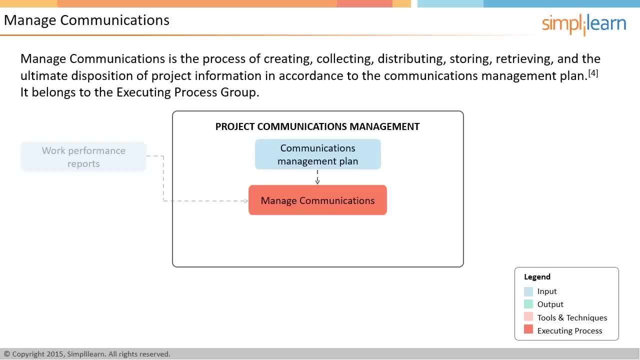 Communications management plan is an important input. Work performance reports have information regarding project performance and status information. organizational process assets are the standard templates created for the status report by organizations. in some organizations there are guidelines for communication distribution. enterprise environmental factors are the other inputs to this process. various 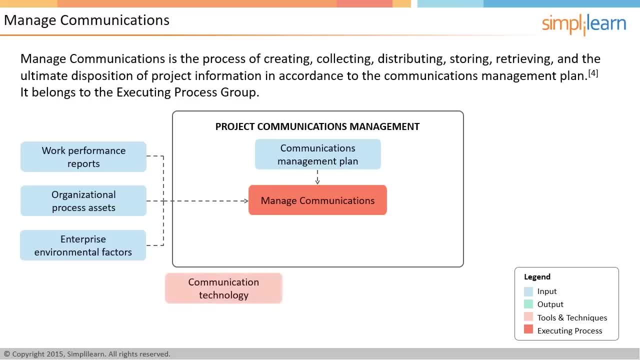 tools and techniques are used in this process. communications technology represents the means of technology that is, email, instant messaging, telephone conferencing, etc. that are used to exchange information. the use of communication models helps you determine the technique that is best suited for a particular situation. communication methods are the various methods used to 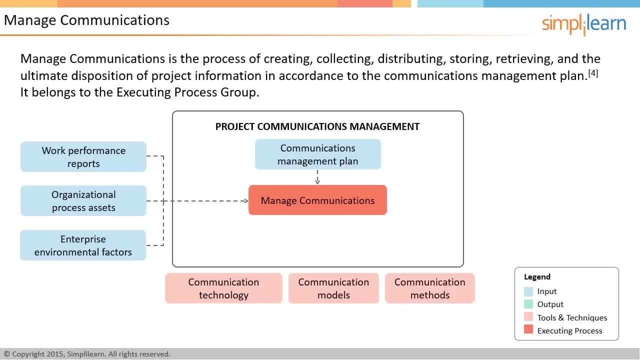 communicate, for example, whether it is interactive or offline, whether information is being pushed by the provider or pulled by the recipient, etc. Information management systems help design a framework for managing the information within a project, that is, how it is acquired, where it is stored and how it is distributed and destroyed In performance reporting. 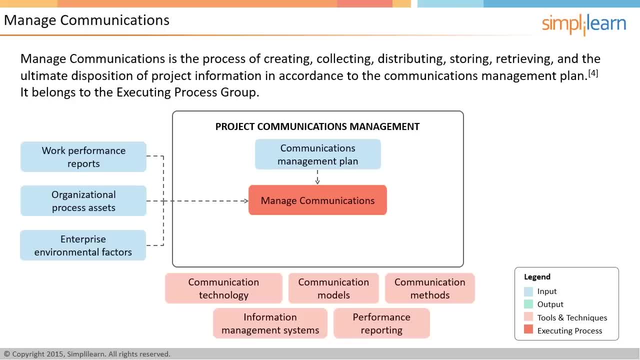 all the information is synthesized in the form of performance reports that are later distributed to the appropriate stakeholders, and forms an important part of the communications strategy on a project. The first and primary output of this process is the communications messages that are generated during the project. The other outputs include project management, plan updates, project. 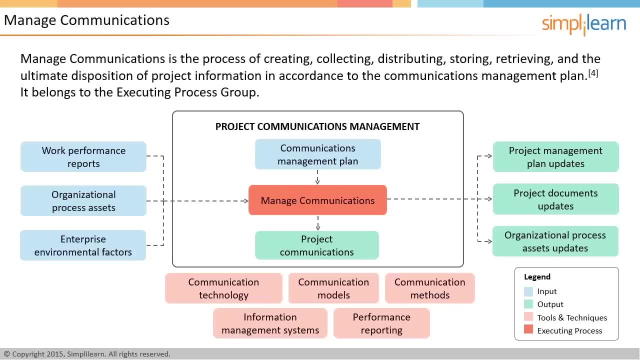 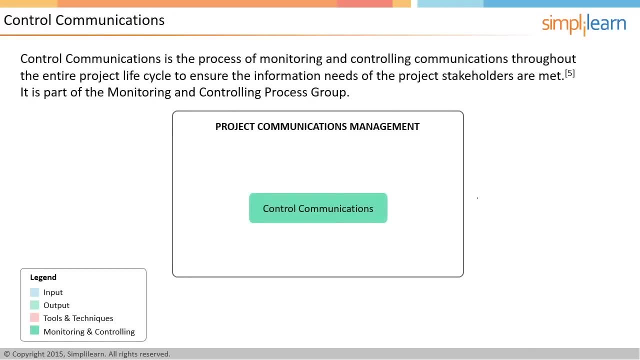 document updates and organizational process assets updates. In the next screen let us discuss control communications process. Control communications is the process of monitoring and controlling communications Throughout the entire project lifecycle to ensure the information needs of the project stakeholders are met. it is part of the monitoring and controlling. 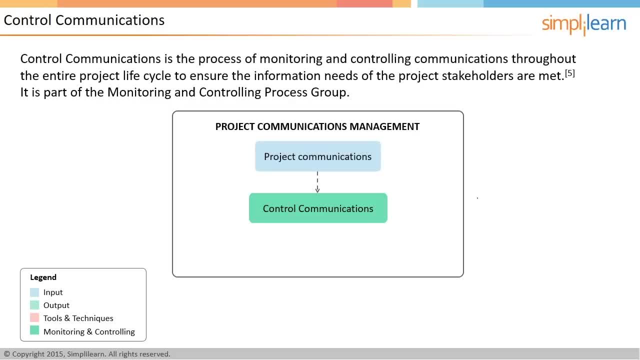 process group. The inputs to this process are the project communications, project management plan and issue log, which has a list of issues that are raised by different project stakeholders, data related to the work being performed on the project and various other project documents, which 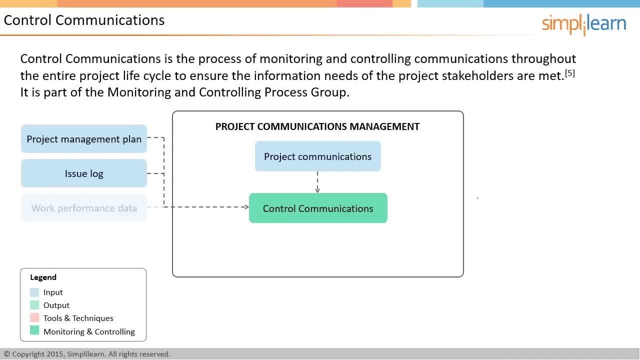 may have to be communicated. Other inputs include work performance data and organizational process assets. Let us look at the tools and techniques in detail. The information management systems provide tools to collect, consolidate and present the information in the form of cogent, concise. 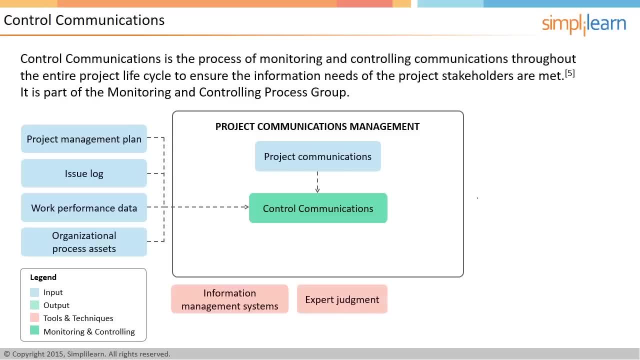 communications. Expertise must be sought from different stakeholders on how you should go about this process. Several meetings may be needed to ensure the efficiency and efficacy of the communications. The major outputs of this process is the work performance information, which indicates that the work performance data has been analyzed, interpreted and presented in an easily. 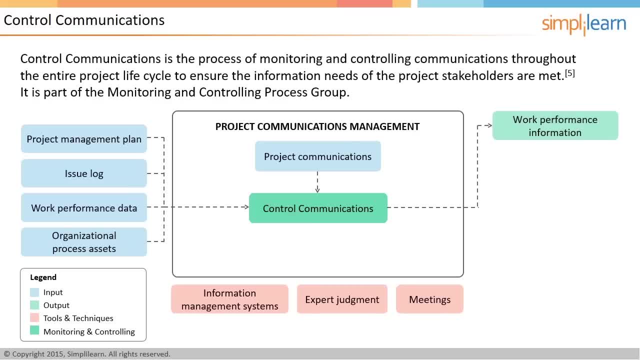 comprehensible form. This process may also give rise to change requests, updates to the project management plan, project documents and organizational process assets. In the next screen, let us look into a business process that is designed to help you better understand this concept After reading the problem statement.